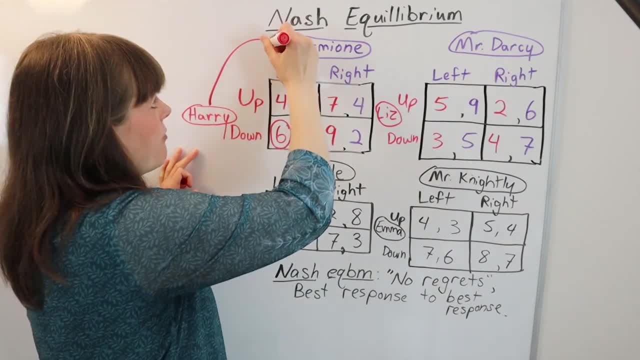 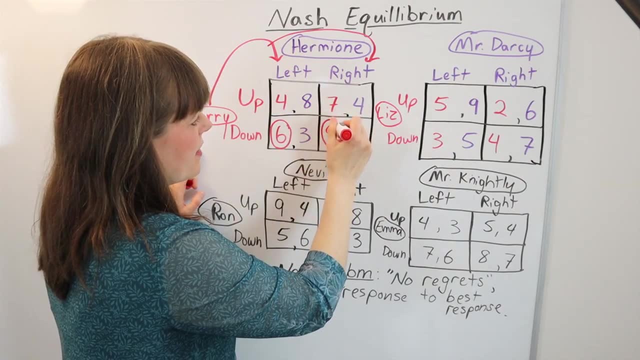 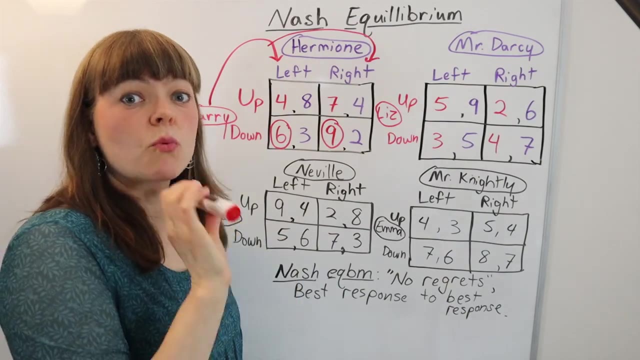 and I prefer the six as Harry. and if Hermione goes right, will I, as Harry, prefer the seven or the nine and I prefer the nine. So he actually has a dominant strategy, meaning his best response is always down, no matter what she does. And then, once we've done Harry's perspective, we're going to 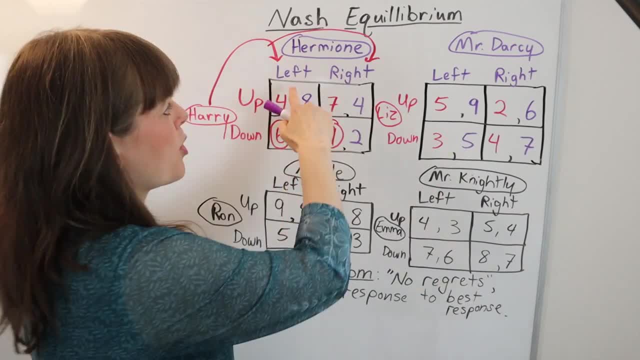 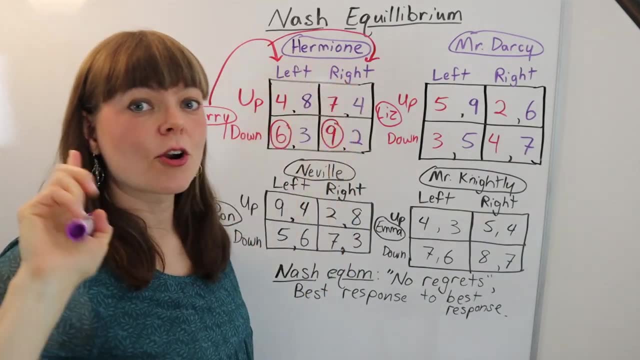 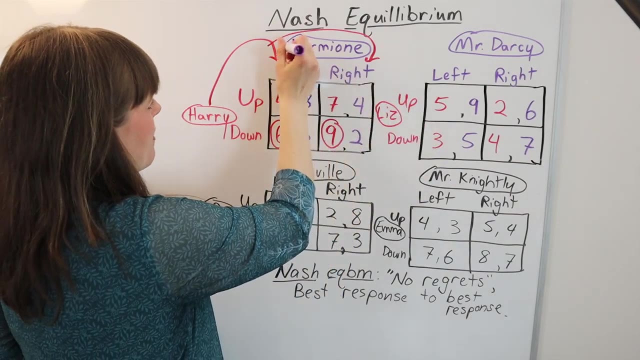 flip perspectives and look at the whole thing from Hermione's perspective, looking only at the second payoffs listed, since she's player two. and yet Hermione is going to check Harry's strategies to say what's my best response. So Hermione comes here and Hermione says, checking Harry's 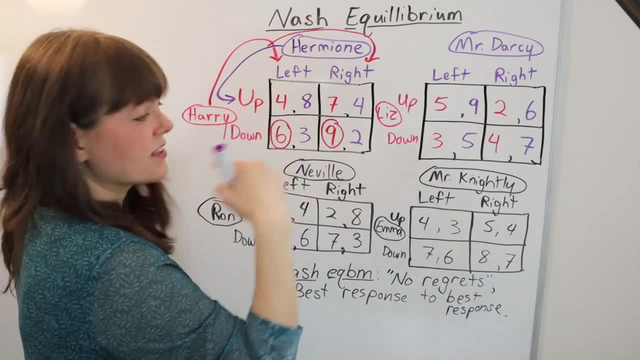 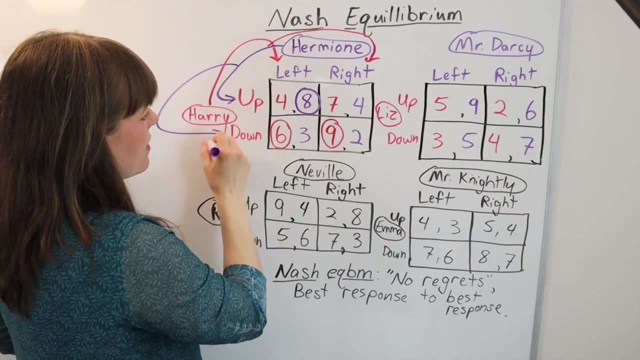 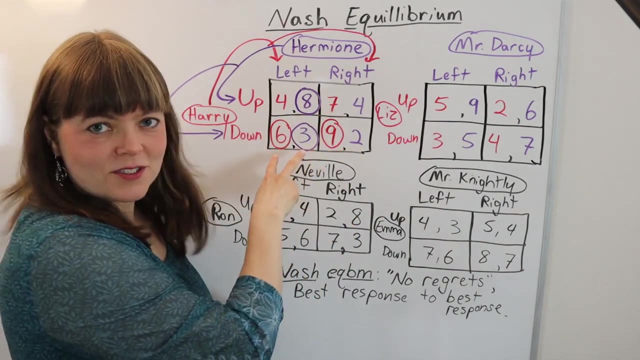 strategies. if Harry went up, I, as Hermione, would prefer the eight rather than the four. and then Hermione says: if Harry goes down, then I, as Hermione, would prefer the three over the two. and then anytime you have two circles in the same box, that means it's a best response to a best 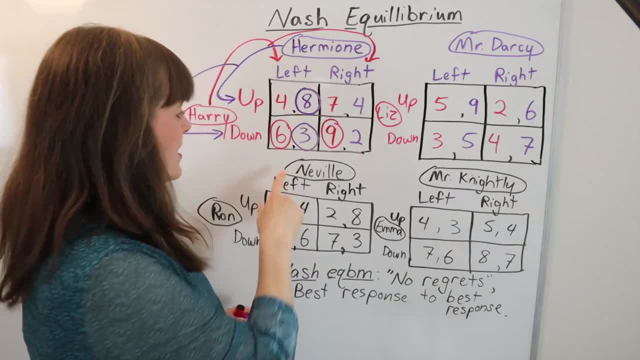 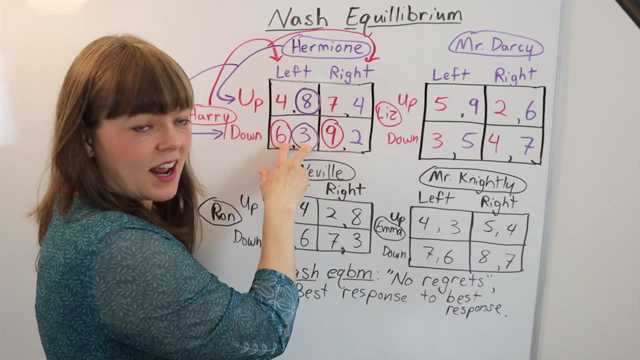 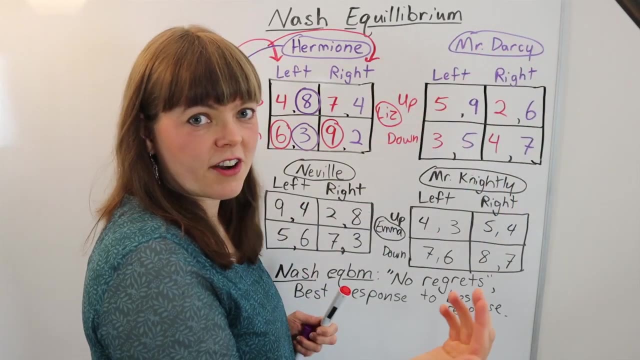 response or Nash equilibrium. Now we notice here that we have an interesting situation because both players would prefer this box up here, but yet this is the Nash equilibrium, and that this is actually a prisoner's dilemma. I won't get into that here, but let's do this next box, Starting from Elizabeth's perspective. we look at all. 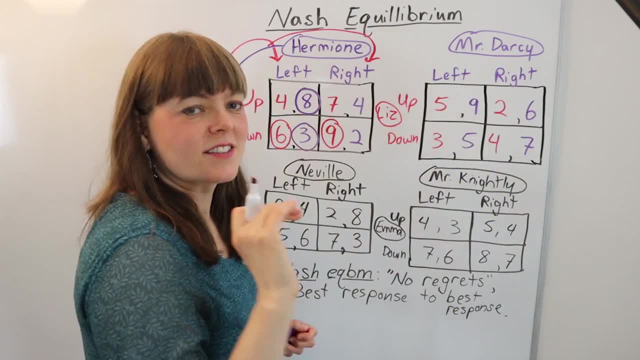 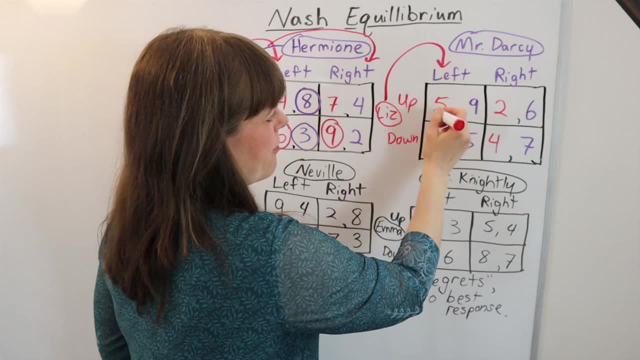 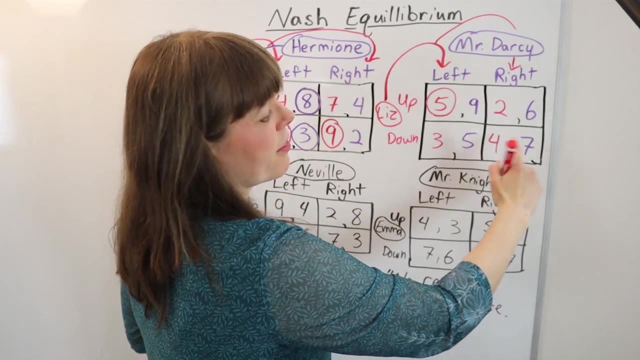 Elizabeth's payoffs. and yet we check Mr Darcy's strategies. So Elizabeth says: if Mr Darcy went left, then I, as Elizabeth, would prefer the five rather than the three. If Mr Darcy went right, then I, as Elizabeth, would prefer the four. 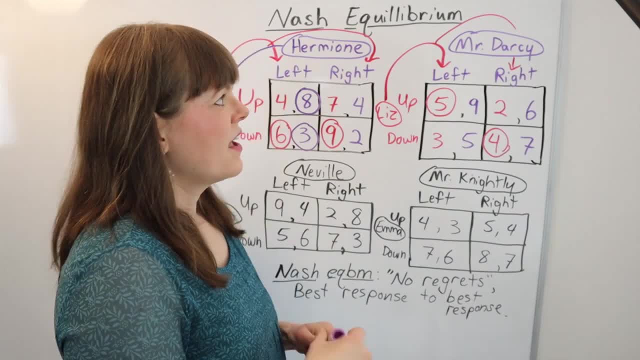 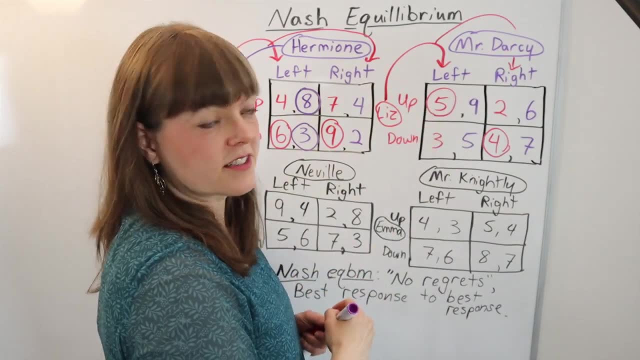 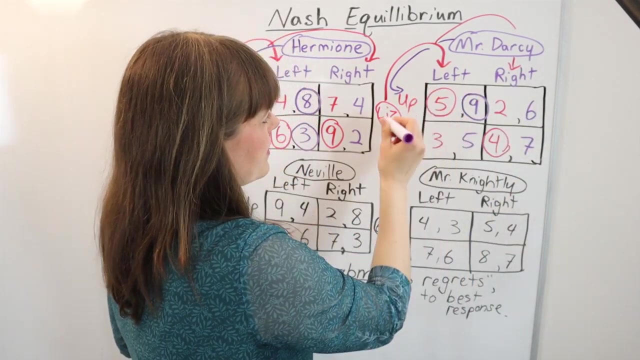 Rather than the two. and then we flip perspectives and think from Mr Darcy's perspective as player two. yet he is going to check Elizabeth's strategies. He says if Elizabeth goes up he would prefer the nine over the six, and if Elizabeth goes down he would prefer the seven rather than the five. 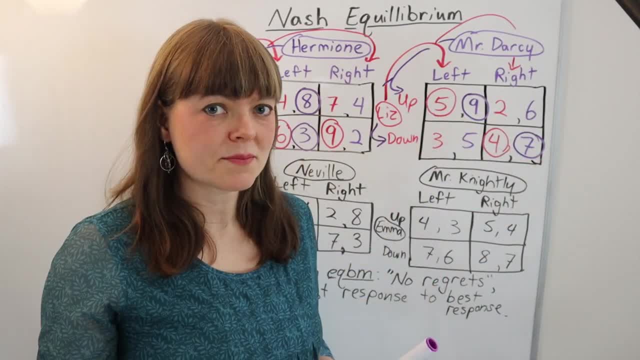 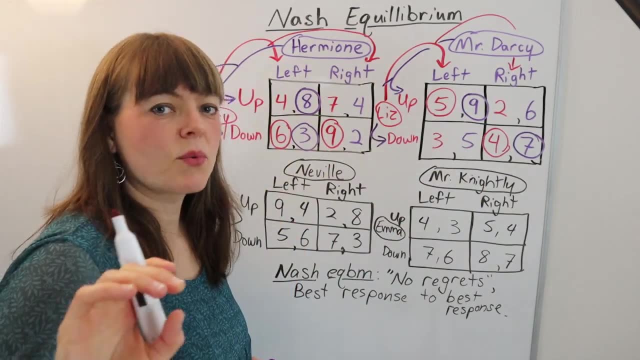 So in this box we actually have two different Nash equilibriums. Now, what if your game is not nice and color-coded like these? well, in that case, I actually have a tip. In that case, sometimes I will underline the, the payoffs to begin with, just to help me organize my my thoughts. So down here, Ron.